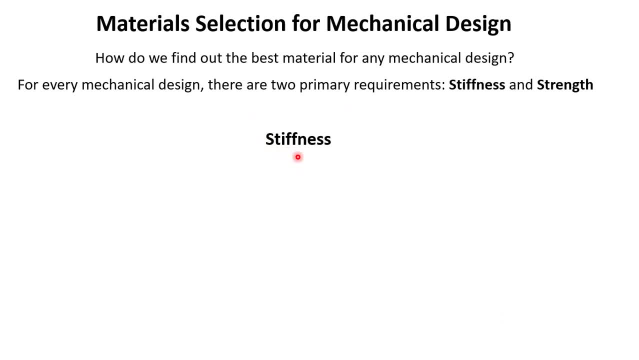 way of selecting a material for the best stiffness. Let us look at this picture: a bicycle. This is a quite old-fashioned bicycle. Still we are using this kind of bicycle. So here, in order to get the right kind of stiffness, many design changes have been done. For example, you can see this is: 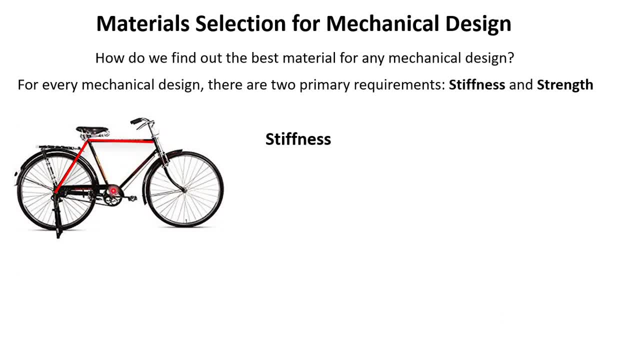 a truss. So basically, a truss is to withstand very high load without much of deflection. So this is a rigid structure. In the wheel we can see there are spokes, and these spokes also have sufficient stiffness so that this wheel does not buckle. Similarly, every part of this bicycle has. 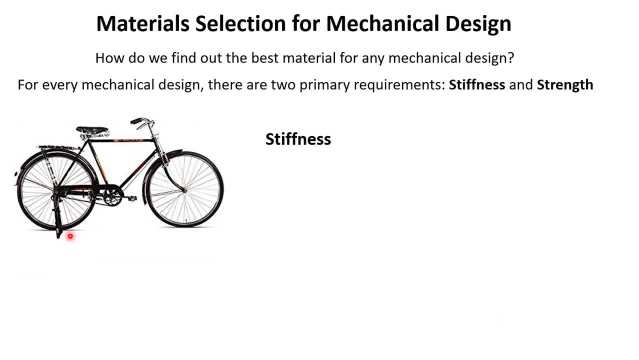 been designed and the material has been selected such that this bicycle is not buckled. So this bicycle can give a very good performance without any problem with stiffness, Because if there is a problem with the stiffness, this bicycle cannot be used, For example, if the wheel buckles obviously. 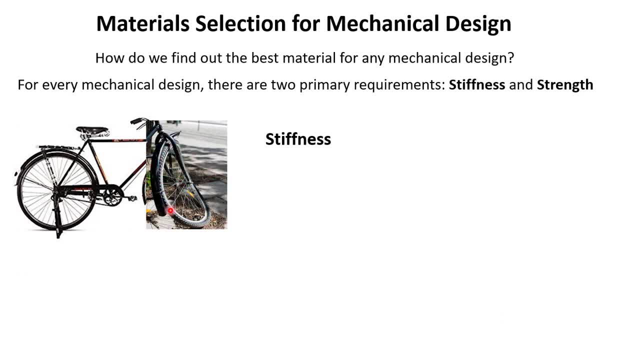 this bicycle cannot be used. Similarly, if if the frame buckles or any part of the metal if deforms during the use, then it cannot be used In this kind of bicycle. you can see that the wheel is not buckled, So this bicycle can give a very good performance without any problem with stiffness. 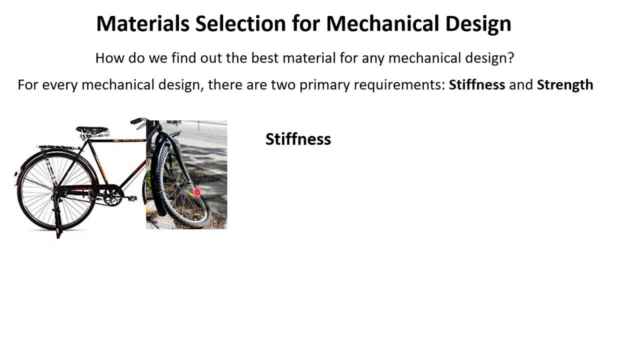 You will see that stiffness has been paid very good attention to, and that's why you will see that these bicycles have become quite heavy. These are quite heavy bicycles and difficult to ride, But from stiffness point of view this bicycle can give very good performance. If we talk about other types, 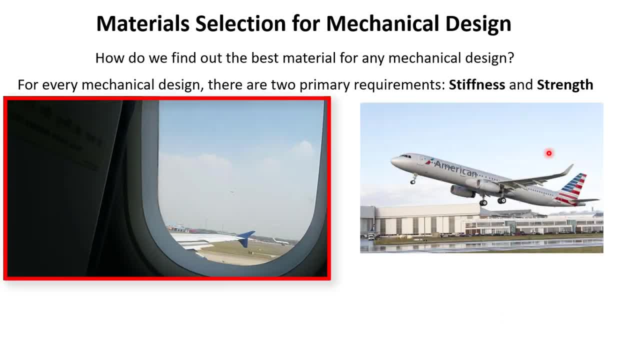 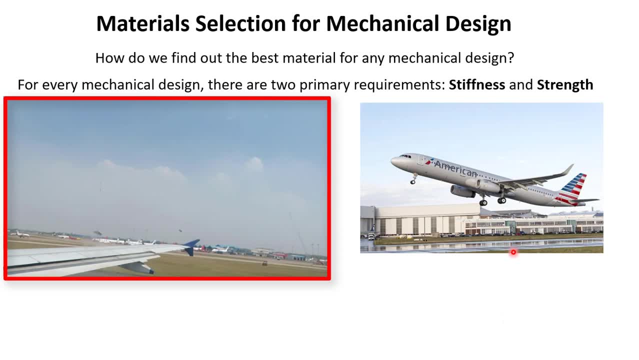 of machines, for example this airplane. The airplane has to fly, It has to leave the ground and it has to fly against the gravity. This kind of airplanes cannot fly unless the stiffness is of the right requirement, Because every part of this aircraft has been designed in such a way that it 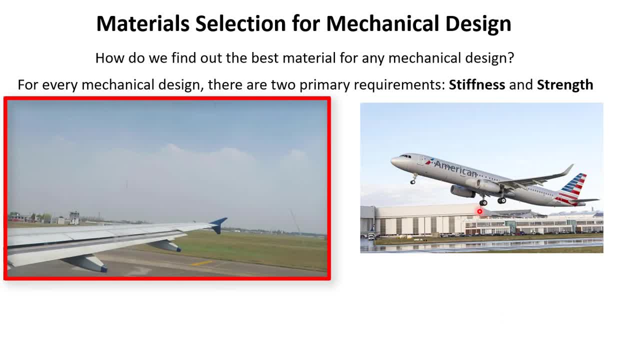 can perform very good in terms of stiffness, And the other requirement for aircraft is, as you know, lightness, For example. the wing must have the right stiffness, It must not be very rigid and, of course, it should not be very floppy. This wing has to have the right kind of stiffness. It can. 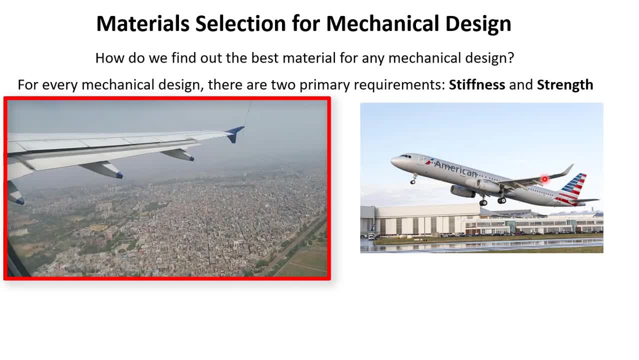 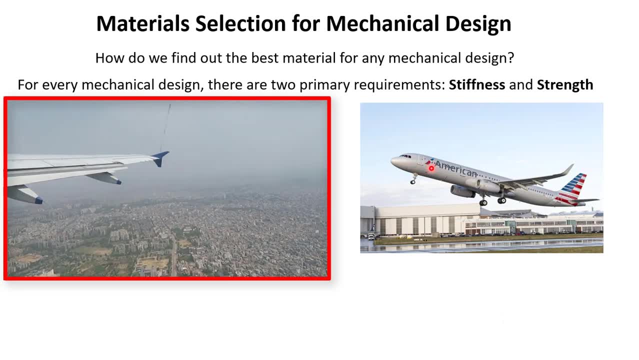 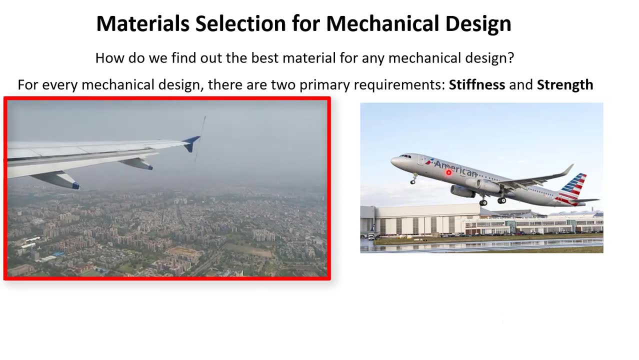 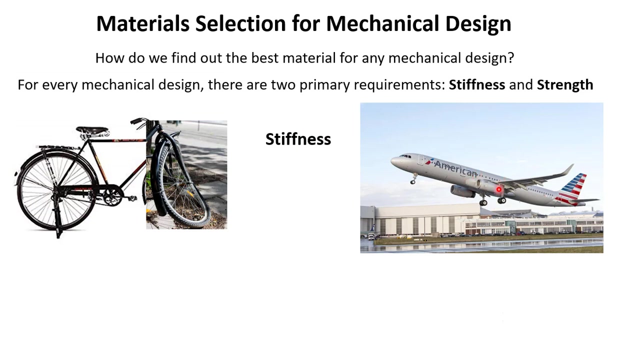 bend to some extent, but not too much. The fuselage part is quite rigid, Quite stiff, Because any movement in the fuselage will lead to some problem in the aerodynamic property of this airplane. Similarly, the landing gears, The engine parts and the tail parts all have to have very required, very precise stiffness, but with 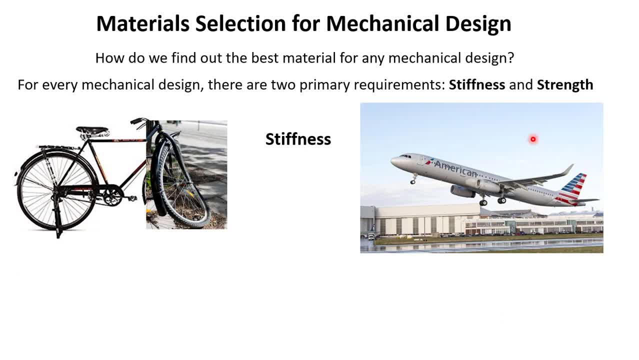 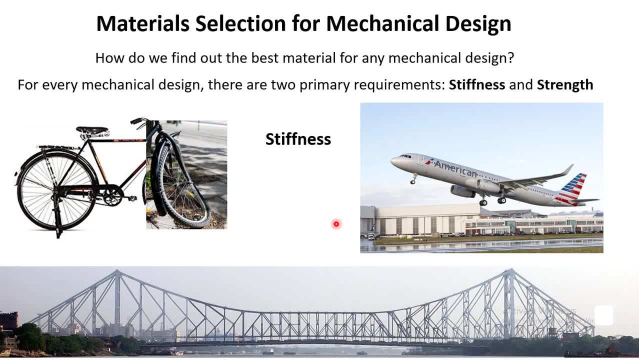 lightness. So this is a special requirement which we did not have to look for in the bicycle, Other kinds of machines or structures, For example a bridge. So this bridge is a cantilever bridge. This bridge has to have stiffness, The required stiffness, because otherwise the bridge will vibrate when the vehicles pass. 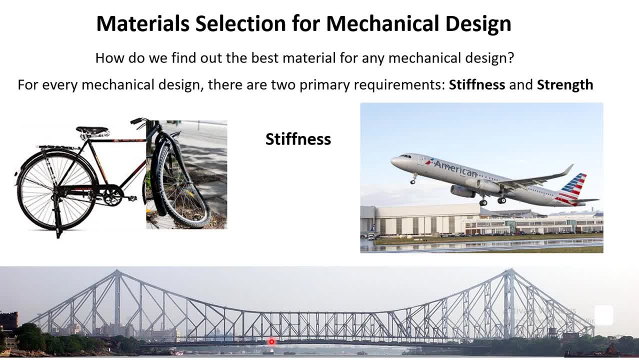 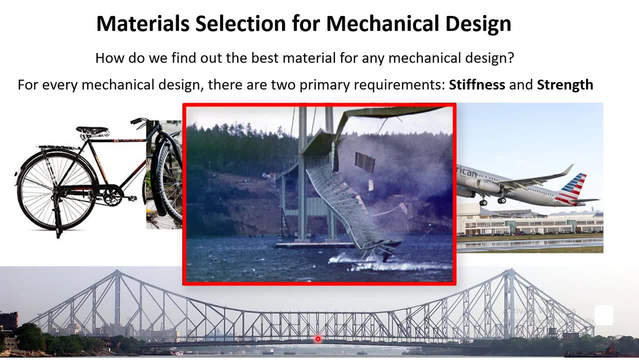 through this bridge And in the case of very strong wind, this bridge will oscillate and swing and may break down. So this bridge also has to have very required stiffness. But with stiffness the bridge can also become very, very heavy, Just like this bicycle we were talking about. 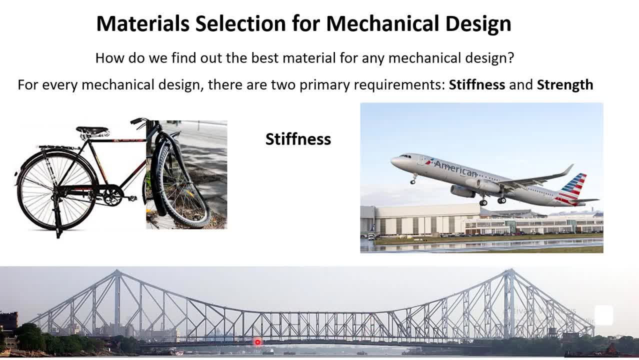 But if it becomes very heavy again, it will not perform the way it should, because a very heavy bridge will obviously will sag because of its own weight. So there is a compromise between stiffness and weight. We want a good stiffness, but we want good stiffness at light weight, For 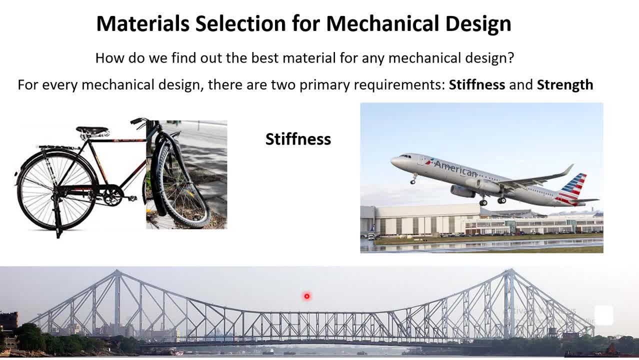 light weight. This is one of the most important part of any mechanical design That we need. The mechanical equipment must have the right stiffness. Lightness in general is an important requirement for most of the mechanical design. The lightweight design concept can provide possibilities of saving materials and energy, which are required in the modern context: Energy saving. 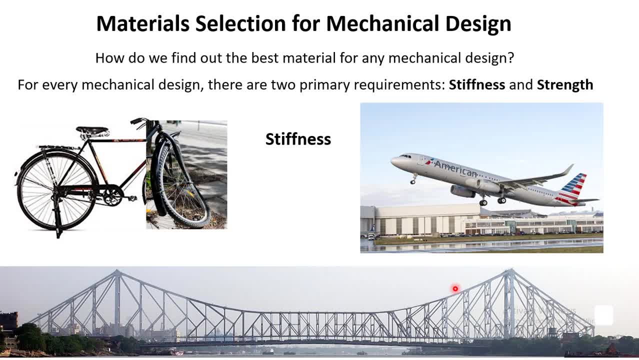 comes from the manufacturing of the product, as less material is needed overall, and also from material efficiency If this product or machine is a mobile one, For example cars, other vehicles such as in railways or airplanes, etc. But with lightness. So we will look at stiff and light. 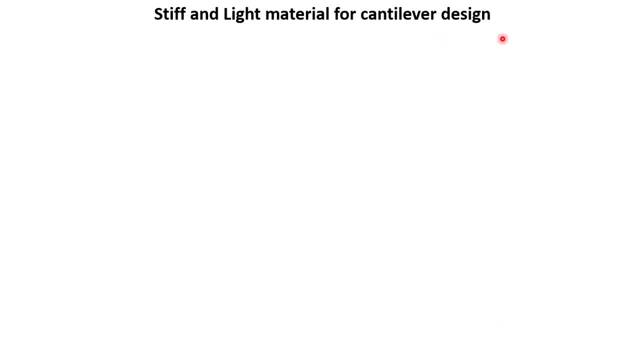 material for cantilever, For cantilever design, And we will try to find out what kind of theoretical analysis we should conduct to find out such kind of material. Obviously, in engineering there are hundreds and thousands of materials available, But we will try to find out what kind of material. 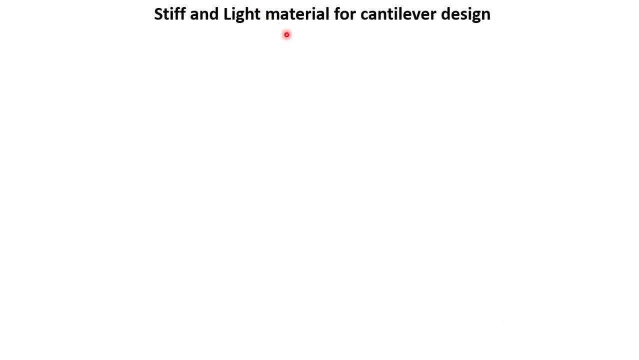 is available. out of these materials, Which materials should I use for cantilever design? And, as you can see that many of the structures that we deal with in engineering do have cantilever type of design. A simple cantilever can be given by this figure. So here this is the cantilever Cantilever has. 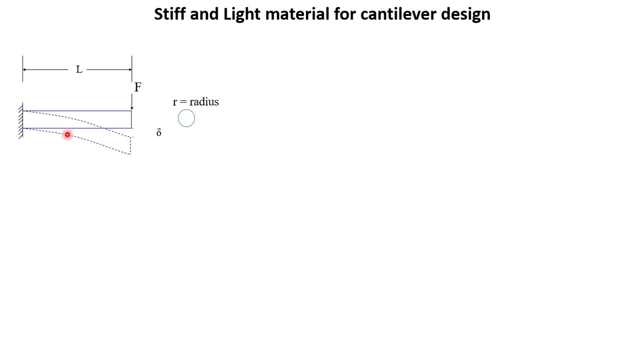 fixed one end and free another end And it has got certain length And the cross-section can be a circular cross-section, or it can be a circular cross-section And the cross-section can be a circular cross-section, And it can be other shapes, For example I section or H section, and so on. 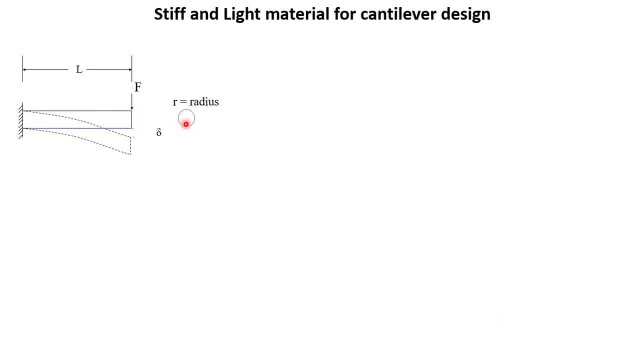 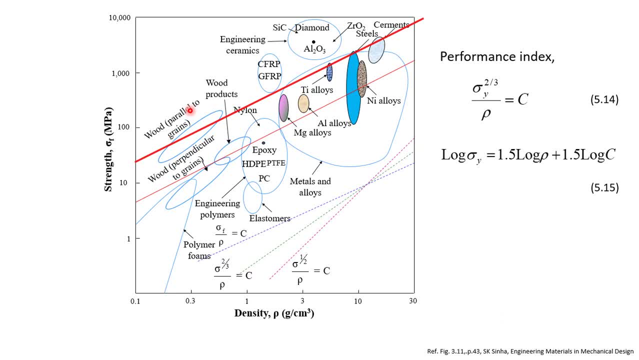 high deflection, So this deflection has been shown here. Slightly high deflection, So this deflection has been shown here. Slightly high deflection, So this deflection has been shown here Slightly. the best material for any kind of mechanical application. In this example we have used 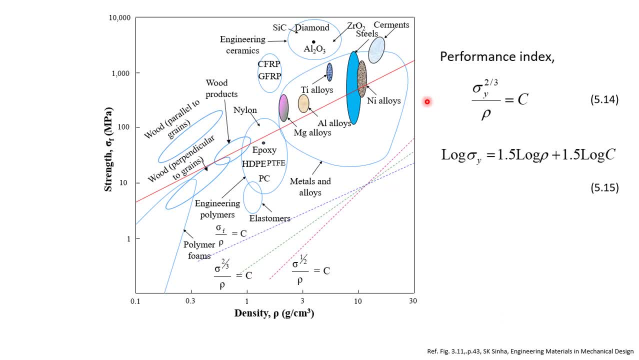 cantilever as one of the structural member. but we can have other kinds of application. We can have tie rod, we can have three-point bending and so on. So in each analysis, this part, the performance index part, will change and depending upon this performance index we can find. 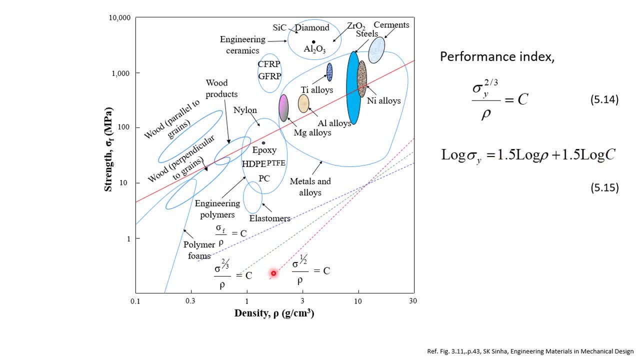 out that this straight line will have different slope. for example, in some cases this will be the slope, while in other cases this will be the slope. So by changing this slope, we can see that the material which will be the best for this application will change to some extent. Now specific modulus. 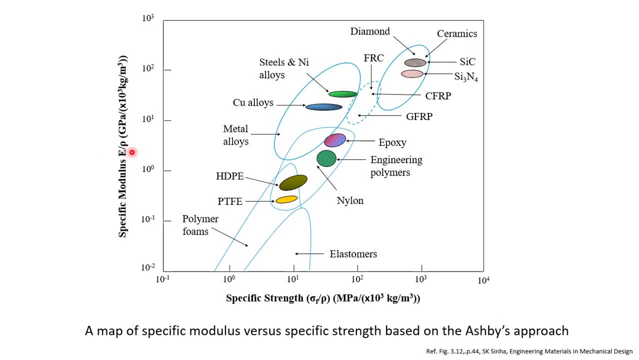 modulus divided by rho or density is known as specific modulus and specific strength. fracture strength divided by rho or density is known as specific strength. So for all materials we can calculate the specific strength and specific modulus and we can plot on this type of graph. So here you can see. 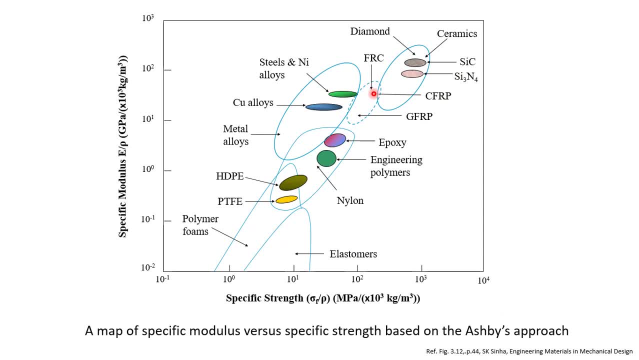 all materials are represented. So these are group of materials like ceramics, steel and other metallic materials, polymers, composites and elastomers and polymer foams. Now, if we find out the best material for best application, we need very high specific strength. that means the material should be very 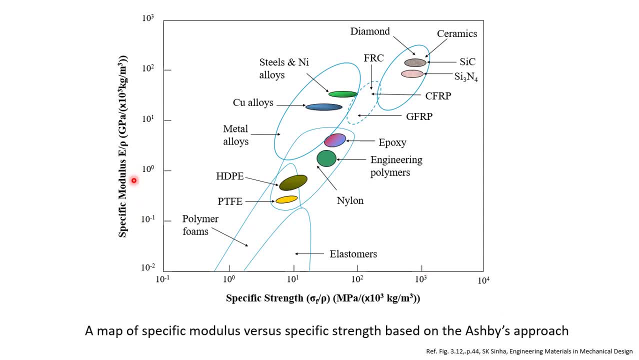 high strength for its weight, and specific modulus should be high as well. So the best material will be in this corner, where we get the best in terms of specific strength and best in terms of modulus. Again, we can see that ceramics are very good high performing materials, but, as I said, ceramics have 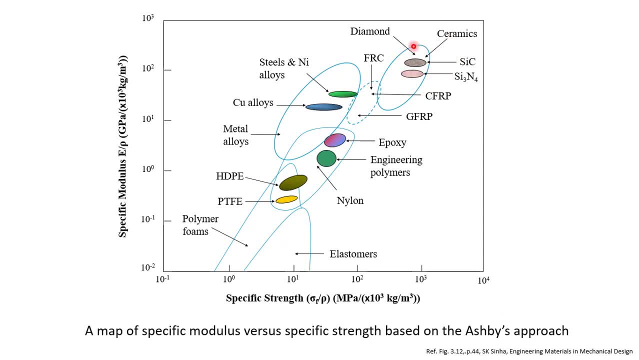 problems with fracture. they are not applicable for tensile application but for compressive application. they are very good materials. After that we can see that steel and nickel fiber reinforced composites- these are very high performing materials. Nickel alloys are also considered very good materials. The plastics are not very good in their pure form, so the plastics can be good material in the form of composites, but in the chance of an high-performance material they work very well. So plastics can be a good material for very high performance, but in nature they do be expensive. możli vilankar h? yumon h? anderlooking esraind? 不�ار 그런데 dikkan paraglumarỉ. 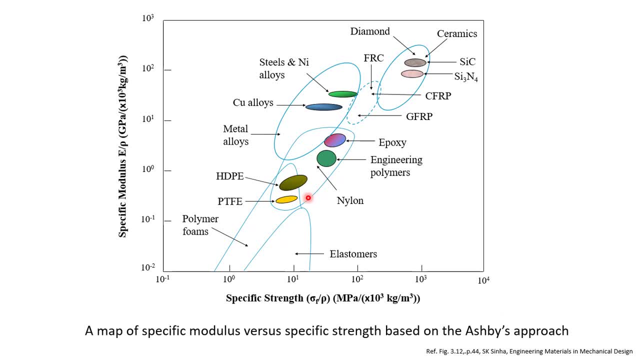 but in their pure form, they are not very good for structural application, where we need high specific strength and high specific modulus. Similarly, elastomers and polymer forms are not very good in terms of these requirements. On the other hand, however, if your concern is to find out, 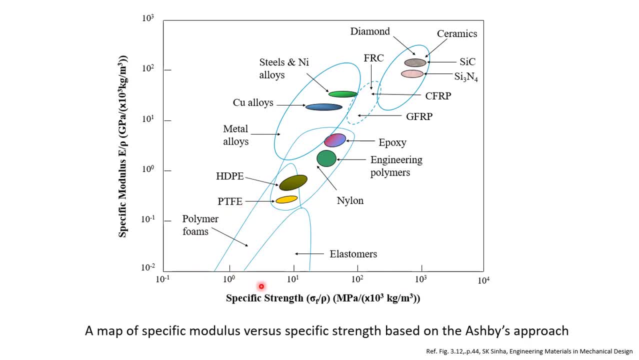 materials which are of lower specific modulus or lower modulus and lower strength, then you might focus on this side. So in this case materials are not of light weight, but some other properties might be more important than lightness. So it all depends upon our requirements whether lightness is. 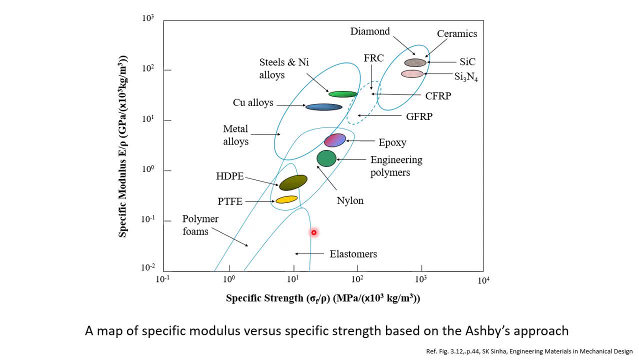 important or not, But for many of the applications, like structural applications or applications where the machine is going to be on the mobile- for example transportation or aircrafts- in this kind of application you will always be focusing on lightness, So in this case materials are not. 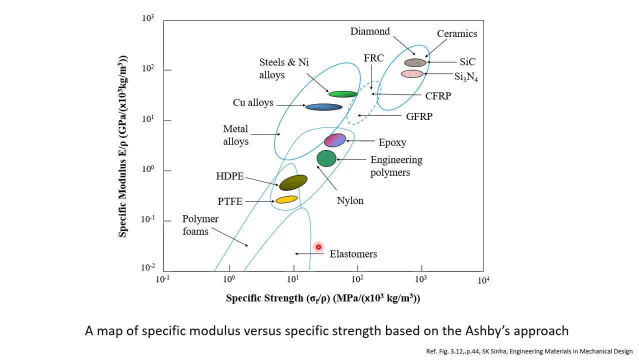 always fine that the materials must have light weight, must be of light weight, So it depends upon our requirements. In this video we have discussed how to consider two important properties like stiffness and strength for any kind of mechanical application, when lightness is very, very important. 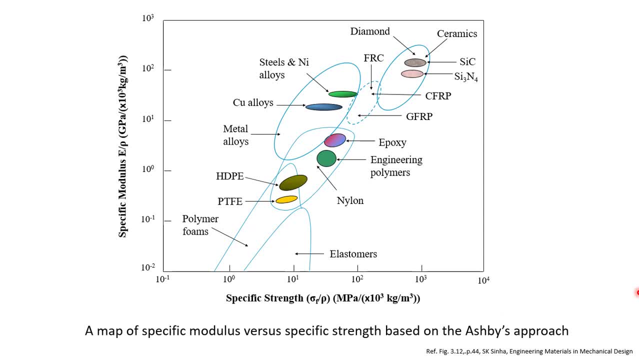 and how we can use Ashby's approach to find out which material would be the best for your application in terms of stiffness and strength. So let's get started. Strength and lightness. Finally, I would like to come back to this example of bicycles I have used. 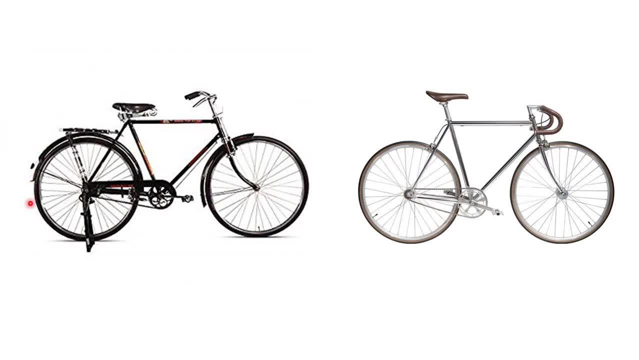 before. So if you see this bicycle, which is old fashioned, and this bicycle which looks quite new design, There are some differences but there are a lot of similarities. As far as the basic design is concerned, they are quite similar. So the truss is still in the same way that has been used in this. 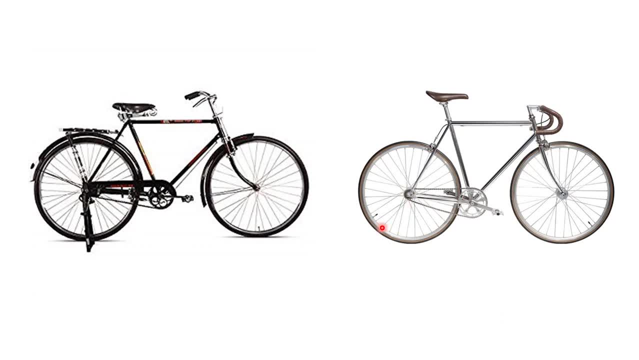 one: The fork, the wheel, the spokes. there are a lot of similarities. But in order to reduce the weight of this bicycle, many things have been removed. So there is no rear rack, there is no the chain guard or there is no fender in this bicycle. So these can reduce the weight, but not much In order to get. 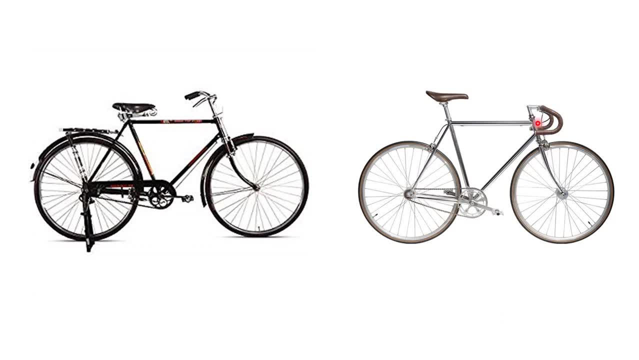 further reduction in the weight. the material has been changed. For this we need to have the efficient design of material, and this is where our analysis of material selection comes into, In order to select the best material which can be stiff, strong but light. So that means it should complete all the 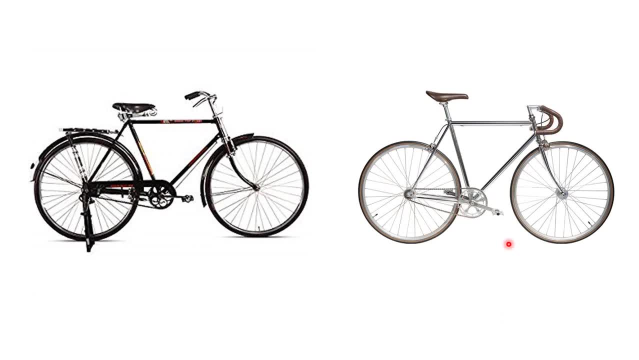 functions. It should provide all the functions with light weight, and for that we need to conduct the analysis and find out the best material. So let's get started. So we have found from our analysis that best materials are carbon fiber reinforced composites, or it can be aluminum or titanium alloys. These are the very efficient material in terms of